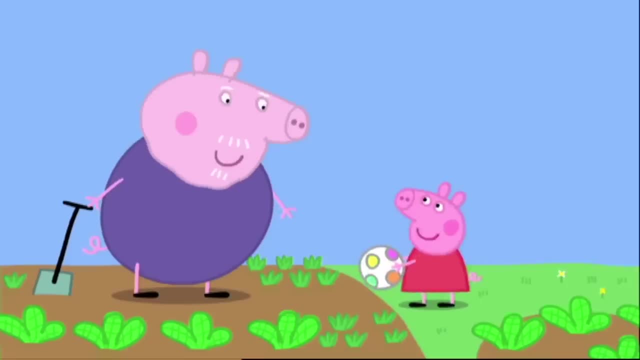 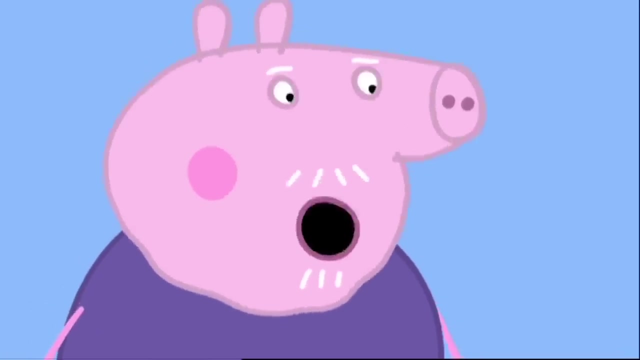 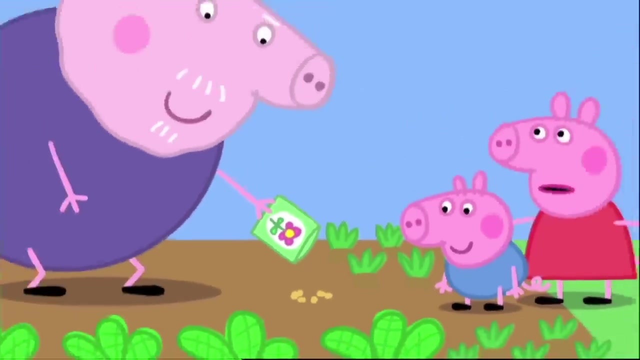 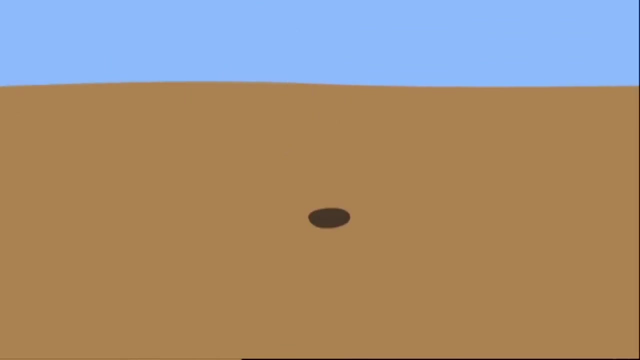 Grandpa, catch, Catch. What's this Dinosaur? A dinosaur, Grandpa, what are you doing? I'm planting these seeds, Seeds. What do seeds? do Seeds grow into plants? I just, I just make a little hole and put the seed in. 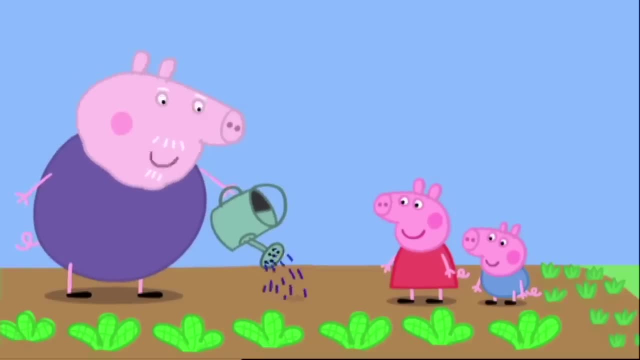 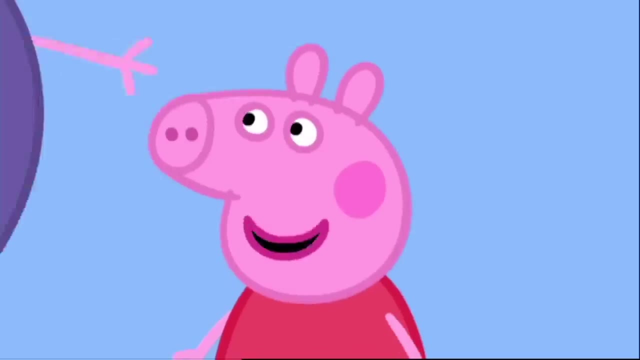 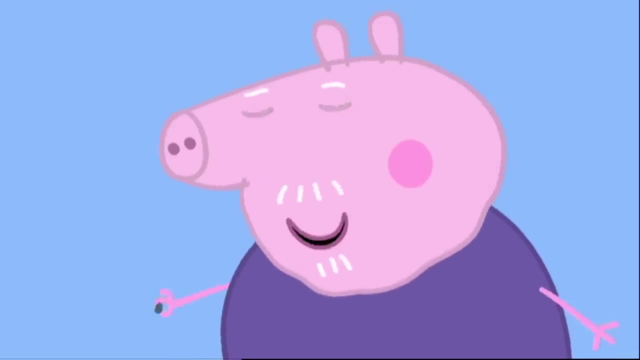 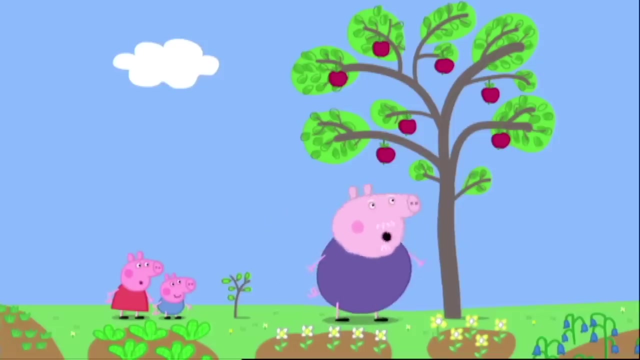 Then I cover it with earth and water it. Everything in my garden grows from tiny seeds like these, Even the big apple tree. Oh yes, This tiny seed will grow into a little apple tree like this. Ooh, And that little apple tree will grow into a big apple tree. 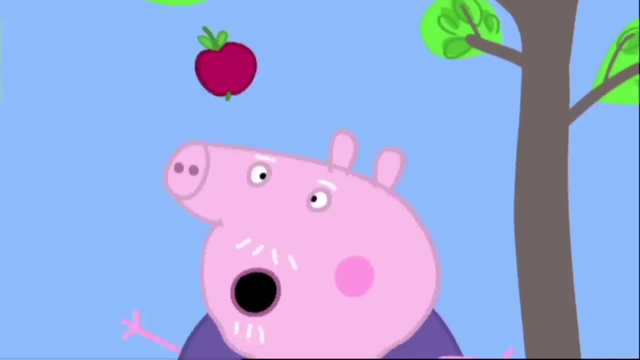 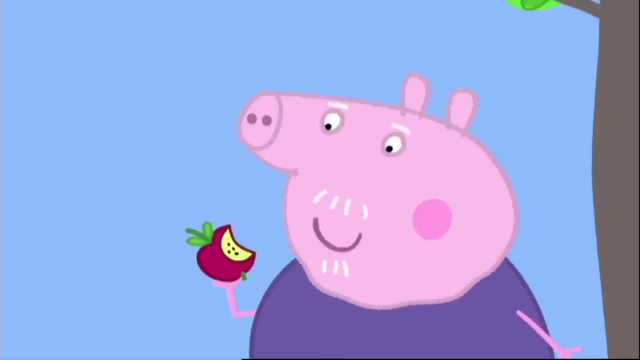 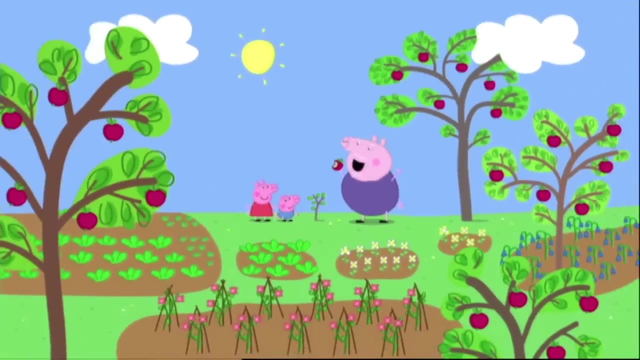 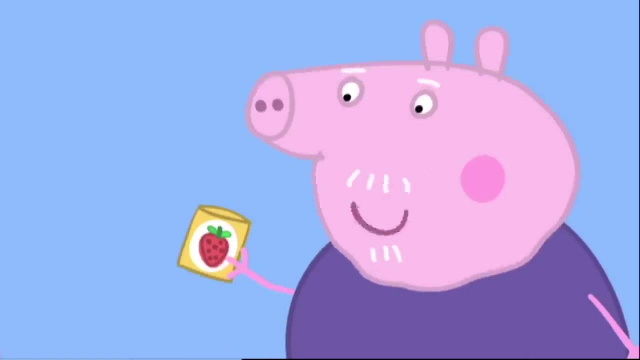 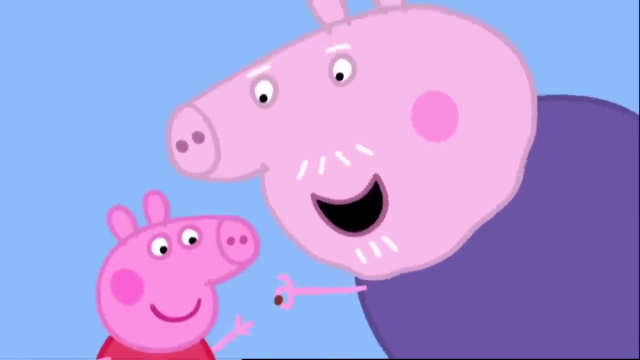 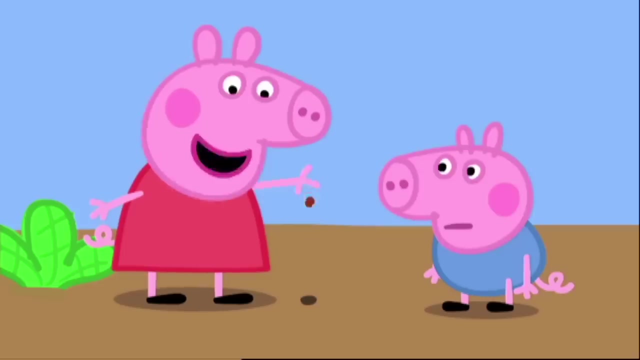 Like this. Ouch, And inside this apple are more seeds To make more apple trees, Exactly, Grandpa. Grandpa, Would you like to plant a strawberry seed? Yes, please, This seed will grow. grow into a lovely strawberry plant. first, make a little hole, shall I water? 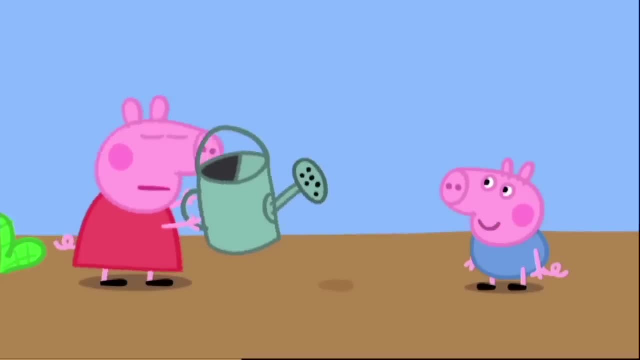 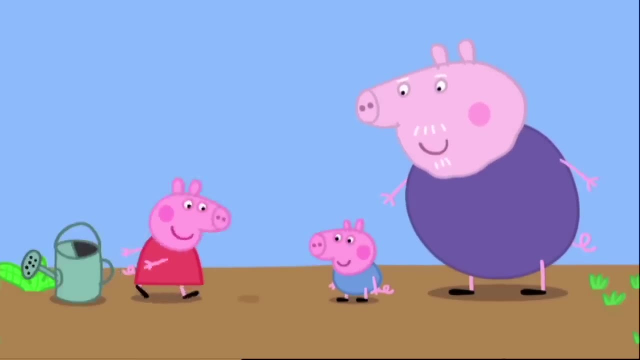 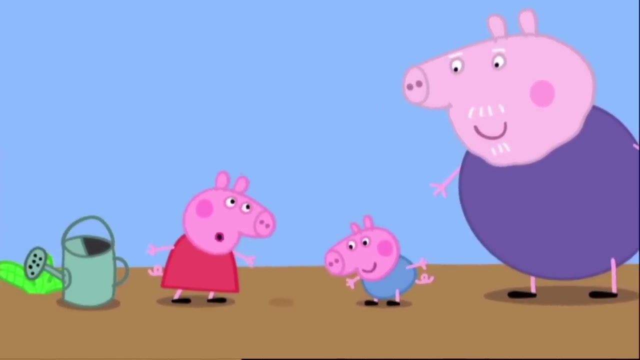 it for you. no, no good. now we wait for it to grow. Peppa and George are waiting for the seed to grow. you'll have to be patient, Peppa. it will take a long time to grow. Peppa, George, it's time to go home, but 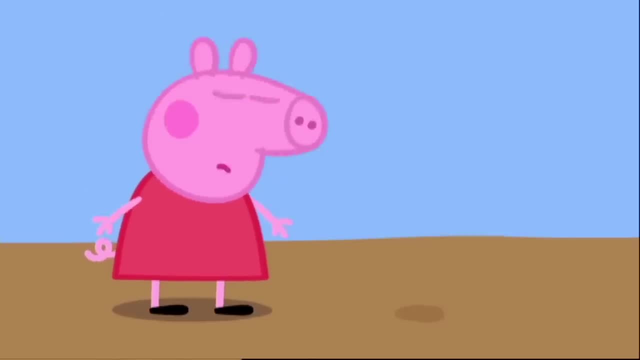 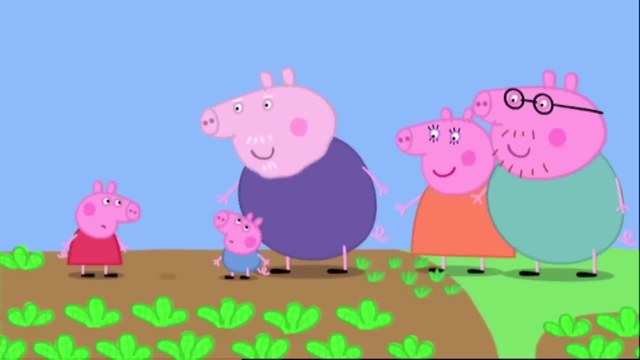 we're waiting for my strawberry plant to grow. I'm just job is for cheese. don't worry, Peppa, next time you come the seed will have grown into a plant. that isn't good for you. now, Peppa and George are waiting for the seed to grow.